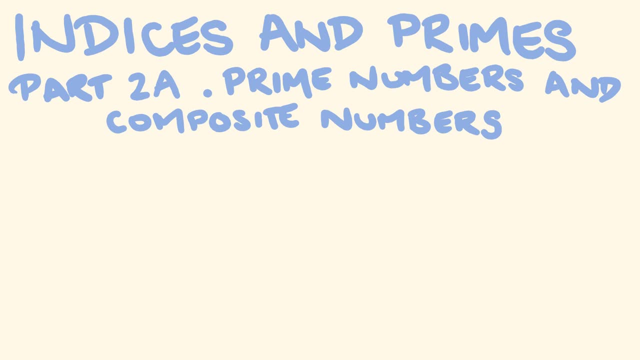 Hello, welcome to this video series looking at indices and primes. In this particular video, what we're going to be having a look at is prime numbers and composite numbers. So let's start with a definition. A prime number is a counting number that has exactly two factors. 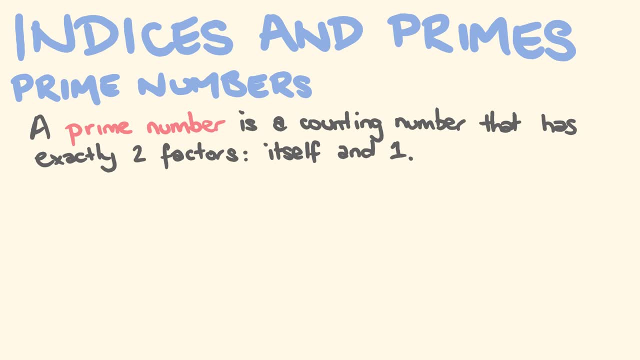 itself and one Now counting number. by the way, these are just numbers: 1,, 2,, 3,, 4,, 5, 6, you know numbers that you count with. So let's have a look at a couple of examples here of some. 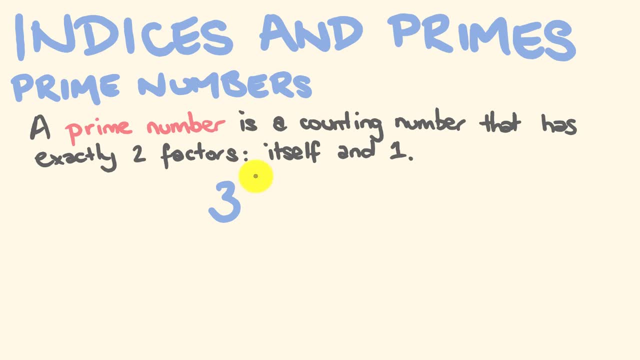 prime numbers. So the number 3 is a prime number, And what makes 3 a prime number is well, the only numbers that go into 3 are 3 and 1.. Okay, because 3 times 1 is 3,. 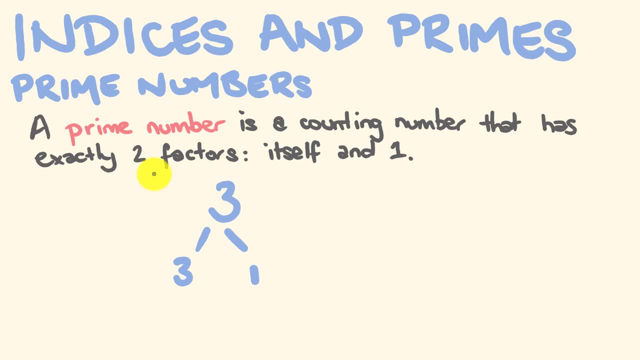 but no other numbers go into 3.. So this makes 3 a prime number. Another example of a prime number is 7.. Okay, because the only numbers that go into 7 are 7 and 1. So another prime number is 2.. 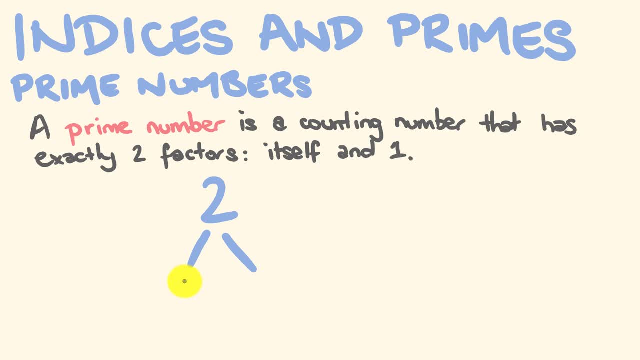 And 2 is a pretty special prime number because it's the only even prime number. The only factors that go into 2 are 2 and itself, and this makes it into a prime number. But you're going to think for every other number, well, themself and 1 will go into it. 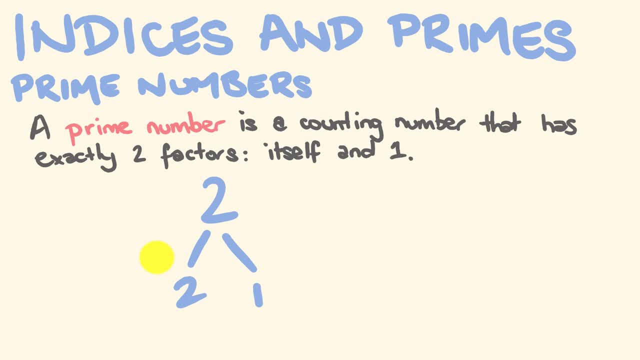 but also the number 2, if it's an even number will go into it. So 2 is the only even number that is a prime number, And you'll see this in a second, when we have a look at composite numbers. In fact, let's have a look at composite numbers right now. So let's now have a look at composite. 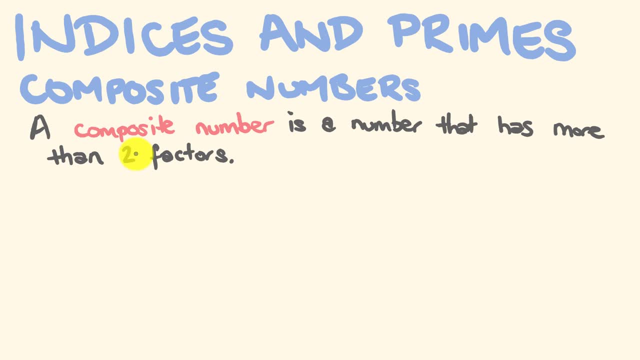 numbers. A composite number is a number that has more than two factors. An example of this is 6.. 6 is a composite number because it has the following factors: The numbers 1 and 6 go into 6.. 1 times 6 is equal to 6.. But we also have two other numbers that go. 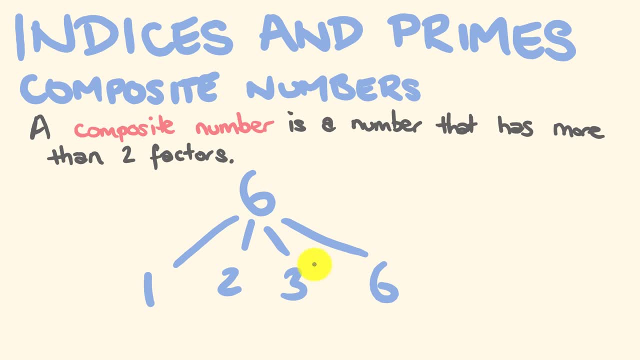 into 6, which are 2 and 3, because 2 times 3 is also equal to 6.. So, because 6 has four factors, 6 is a composite number And you can also look at it as I was saying before. 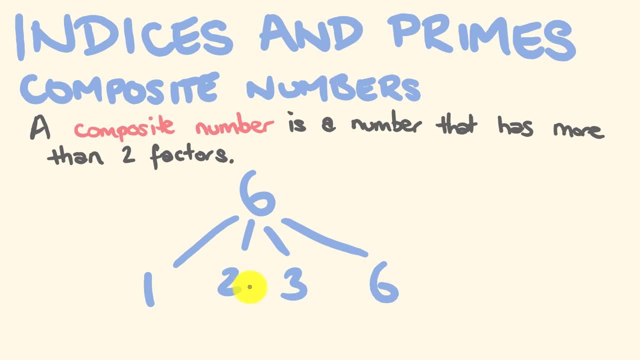 6 is an even number, that's not 2, and we straight away know that 2 is going to go into it. So we can also know that little clue there, that 6 is going to be a composite number. What about we have a look at another example. 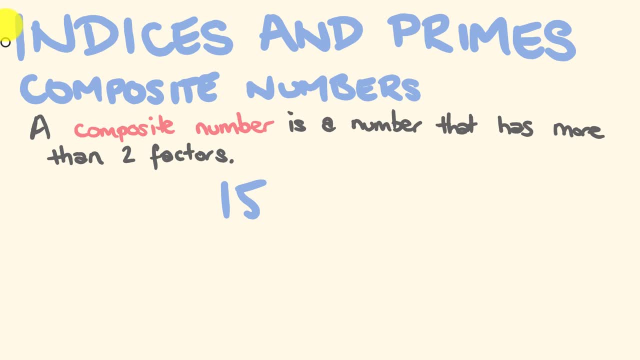 What about the example of 15?? Now, 15 is a composite number. It has the following factors: 1 and 15. But the other numbers that go into 15 are 3 and 5. Because it has more than two factors. 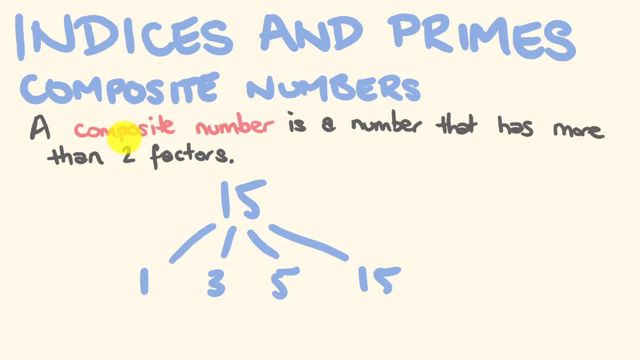 15 is also a composite number And just a little hint here: when you're looking to see whether a number is prime or composite, you can also look at the number 15.. And you can also look at the number 12, and what the number is prime and what the number is zero, Because 25 seems to be a 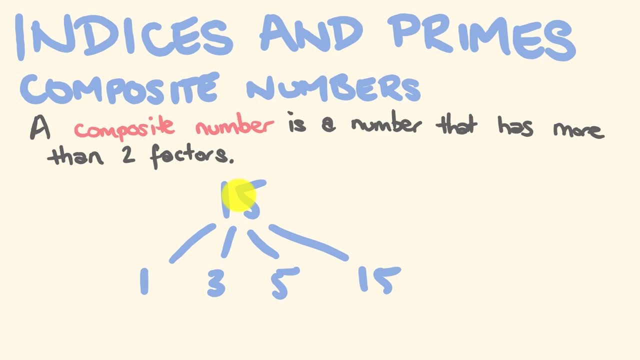 lower number. Anyway, 75 is a divisible political number, so it's going to be a bigger composite number. It's not going to be 5.. Let's also put there 5 to 0. So there are still numbers that go into here. 5 and 0 are not. 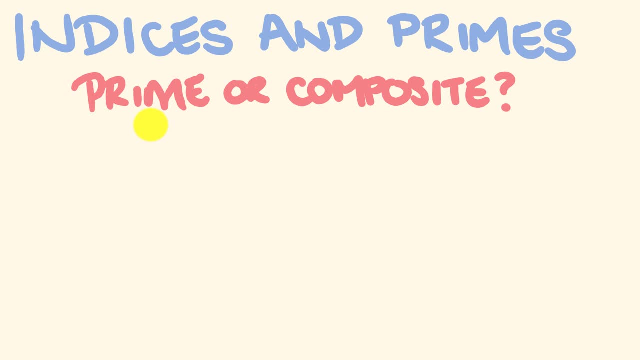 triples. but 5 and 0 are a yes number And by now we can culturally understand what we're looking at here. in future videos 4 and 2 look good numbers, But if 5 and 0 are not numbers, these following numbers: prime or composite? So let's have: the first number is 11.. Is it a prime? 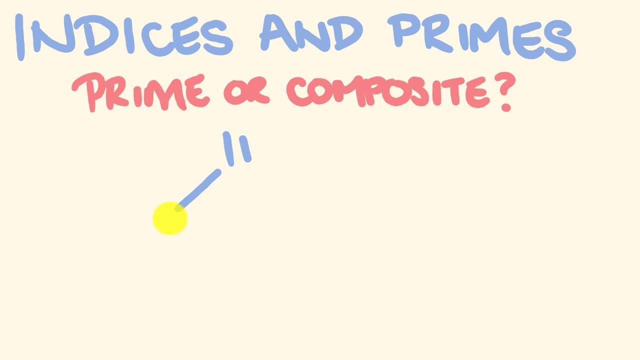 number or a composite number. So what factors does 11 have? 11 has the following factors: 1 and 11.. Because it only has two factors, it's going to make 11 a prime number. Hopefully you got that right. What about another example? What about the number 12?? Okay, what factors does 12? 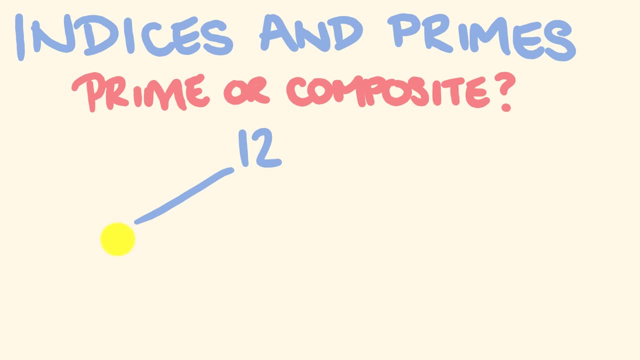 have. So 12 has a whole bunch of factors and you'll probably think of these really quickly. We have 1 and 12, but we also have the numbers 2 and 6, because 2 times 6 is equal to 12. But we 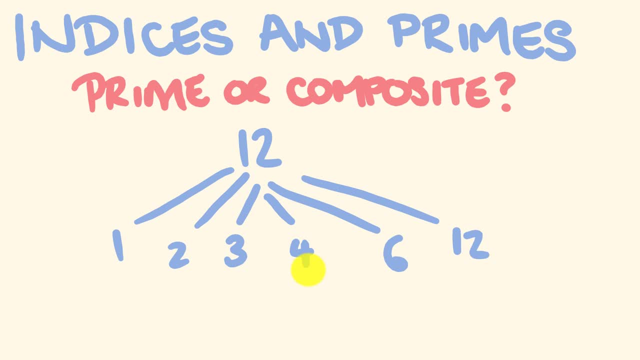 also have the numbers 3 and 4.. So we know that 12 is a composite number. The other thing which might have given this away is because 12 is an even number, that's not 2. we also could have said pretty much straight away that 12 was a composite number. 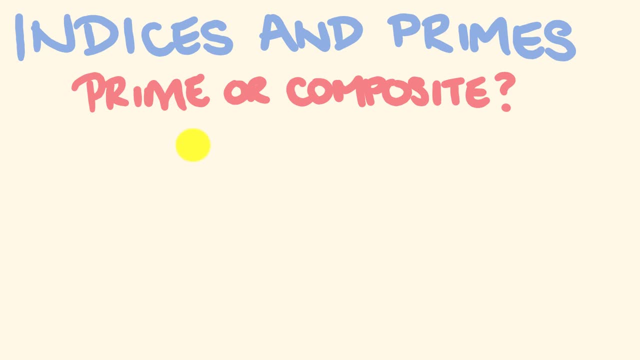 What about one last example? What about a really hard example? now, What about we go the following number: 1032.. Is that a prime number or a composite number? So you can look at this straight away and say: well, we know that this is a composite number, and what tells us this, without working out any of the factors? Because